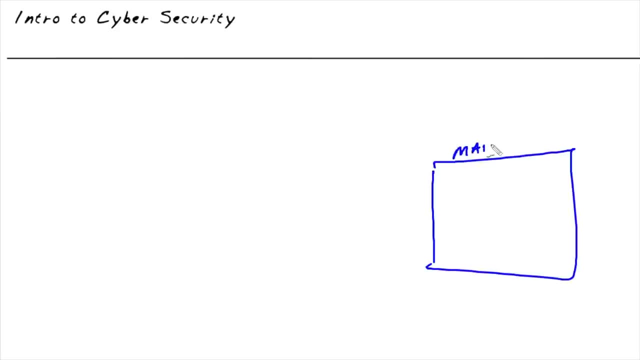 In the early days we had closed systems with old legacy systems like mainframes, with very limited access. It was centrally managed and there wasn't just easy access into the network to get to the mainframe. We came in through a terminal And, as a result, there wasn't that many possible attack vectors or methods, if you will, that could be used to access that data illegally or unlawfully or compromise that data. 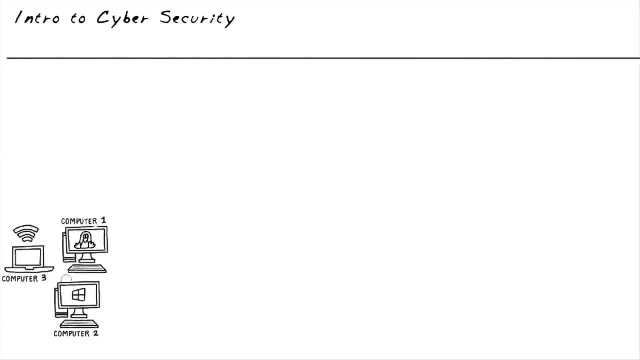 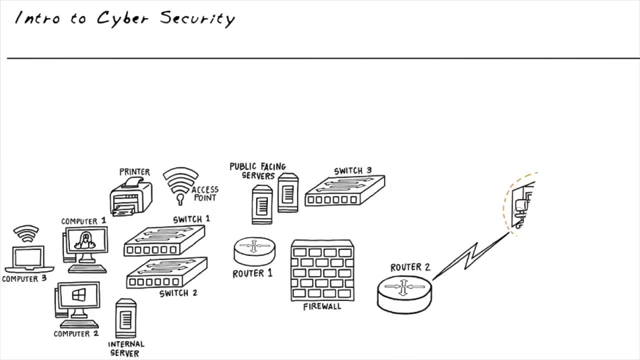 But in the 80s, as we started networking and connecting devices together, the network became more and more available, first with wired local area networks- LANs- and then with wireless access with things like Wi-Fi. It simply made it easier for individuals to connect both honest and innocent users as well as malicious individuals. 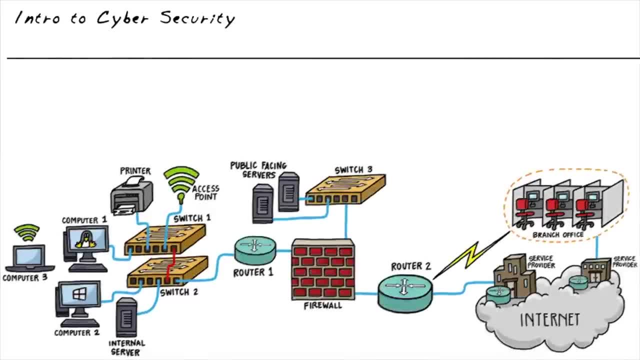 Also, instead of having centralized servers, we now have ba, have distributed devices. we have computers with processing power, we have servers with processing power. we could have servers in the cloud. so having our content and services spread across multiple devices also allows more potential attack vectors or methods for compromise of those systems. another big 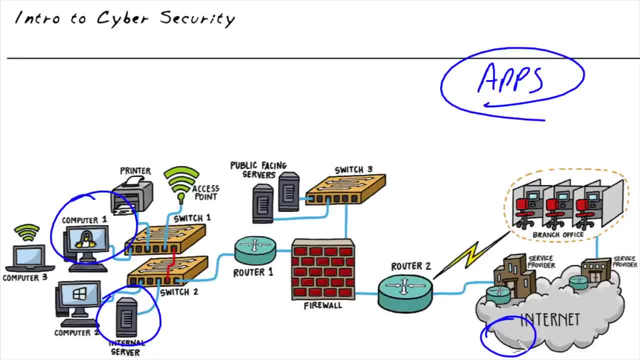 challenge are applications. so we might have a user- let's put Bob out here, so we may have Bob that's using an application- then that application is then accessing data on a back-end server somewhere. but if that app is not secure, that allows additional vulnerabilities to exist where some unauthorized individual could. 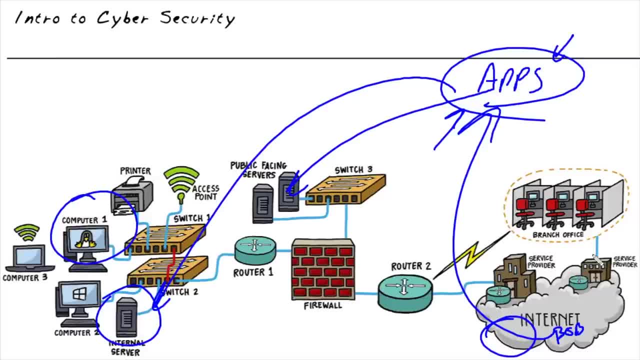 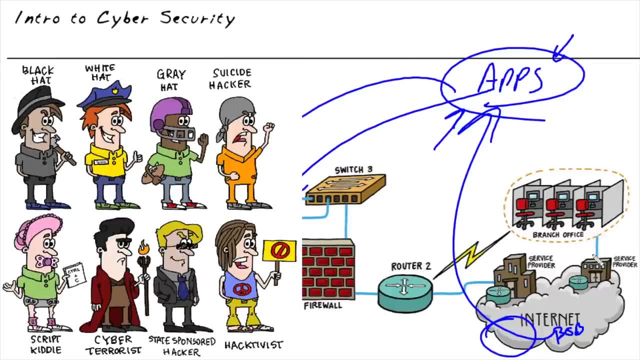 compromise or access our data. and as far as attackers go, the attackers out there are in the millions of potential attackers, and I'm sure that hundreds of thousands of those attackers are actually really, really good at what they do, and that's why it's important for organizations and governments and 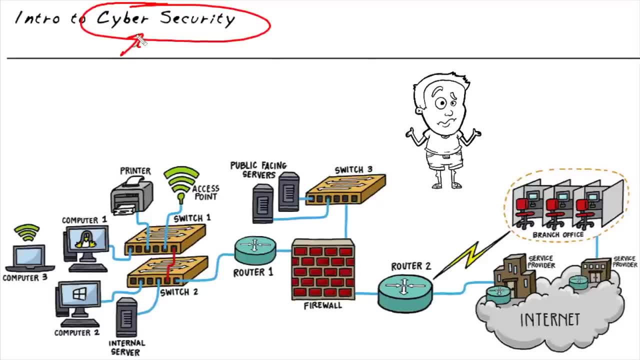 individuals to be really good at cybersecurity. now the question may come up, Keith, what is cybersecurity effectively? it's us protecting our systems, our networks, our applications from any kind of digital attack or compromise, and the reason is so important is because it's so expensive if there is compromise to our systems. 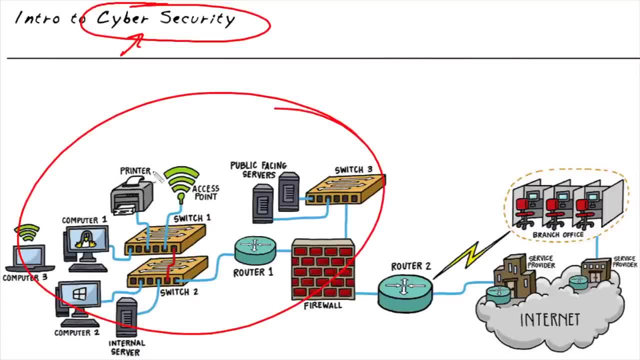 into our networks, into our data. case in point, we may have an organization that spent a decade in building their business and putting other systems in place. they may have hundreds of employees, but if they are attacked and compromised and all the data they had regarding clients and personally, 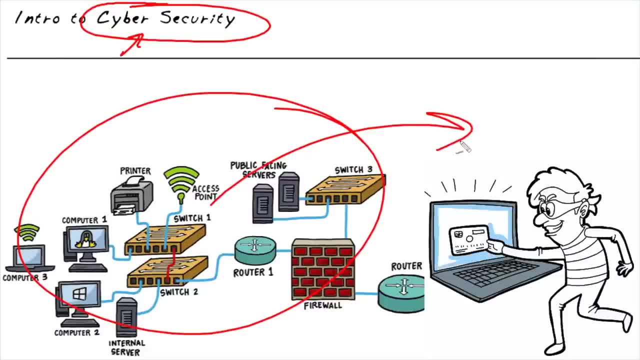 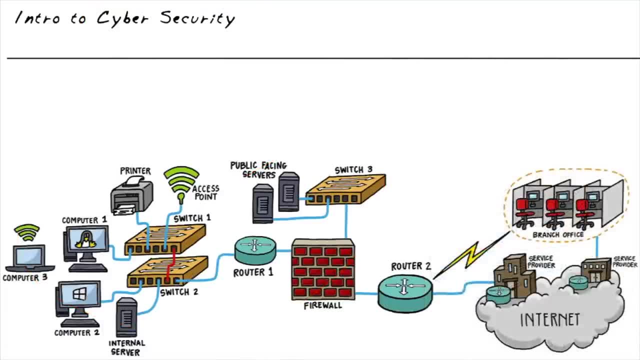 identifiable information and other company secrets. if that's all stolen or exfiltrated out of the company, that may be the end of the company from one simple security breach. and let's pause for a moment and think to ourselves. okay, what does a company or organization really need regarding security? and I think it boils down to 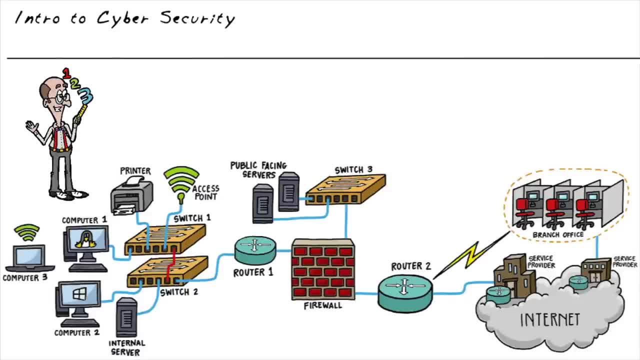 three basic things. number one is that only the people who are authorized, who are supposed to be able to access and see and modify the data, only those people should be able to do that, and to make that happen, we're gonna have to use good authentication, which is identifying. 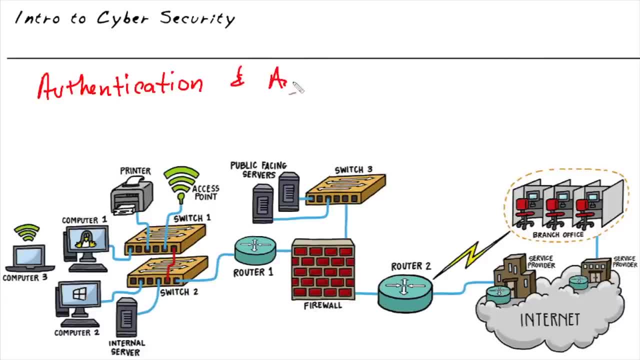 who an individual is or entity is, as well as authorization, controlling what they're allowed to do. and we're gonna do that with technical controls. we're not just gonna do the honor system, you know, only login if you're supposed to. we're gonna force that with controls called technical controls that make sure that. 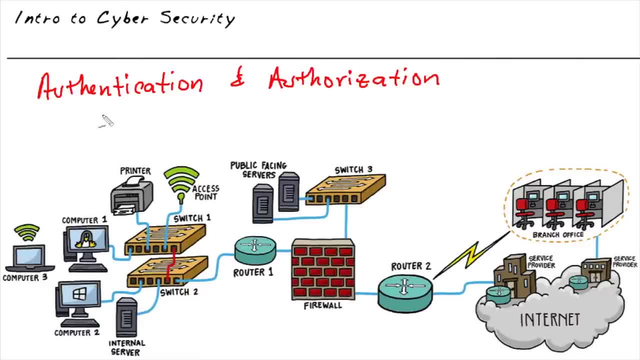 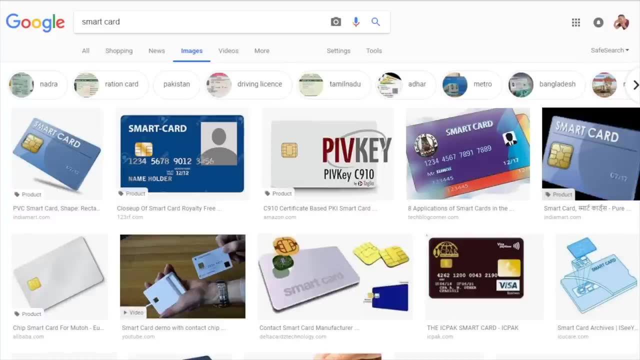 when Bob's logging in, it's really Bob, and some methods that we might use for authentication include two-factor authentication. an example of that is something that Bob knows like a pin or a password, along with another factor, another element such as something Bob has like a card, a smart card that might have a computer chip in it or a digital. 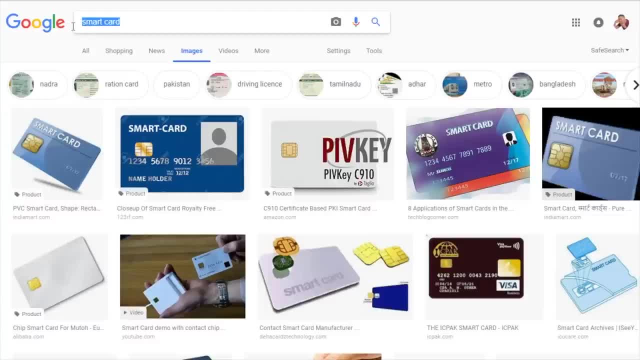 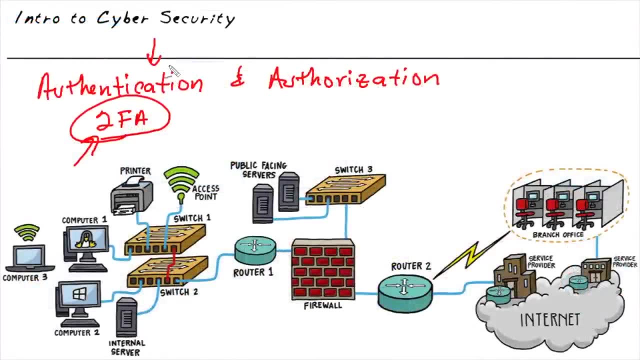 certificate in it And both of those elements, both of those factors, if you will, are required for Bob to log in- And that would be a good example of doing authentication- to prove that Bob is really Bob. Then, once Bob logs in and proves who he is, based on his permissions and 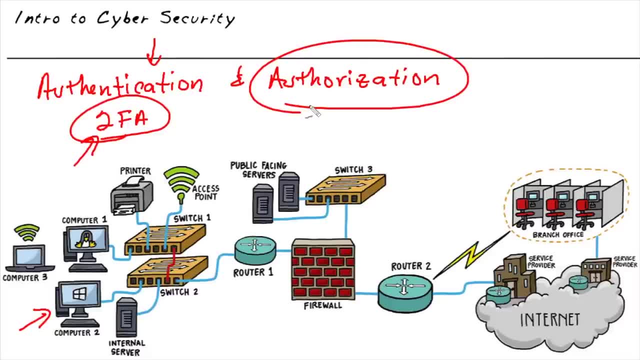 rights. he can access various resources based on his authorization, like permissions of what Bob's allowed to do. Another security goal would be to make sure that the unauthorized people shouldn't be able to see our sensitive or private information, And the challenge is our information. 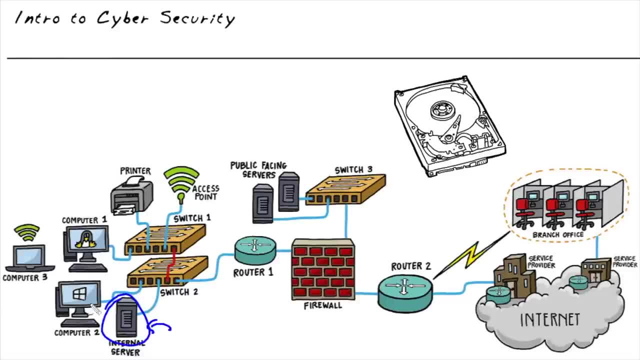 can be lots of places. It can be sitting at rest on a disc or a flash drive, or it could be moving through the network, coursing through the veins of our network, and that would be referred to as data in transit. And if somebody steals a hard drive or if they start listening in on the network, 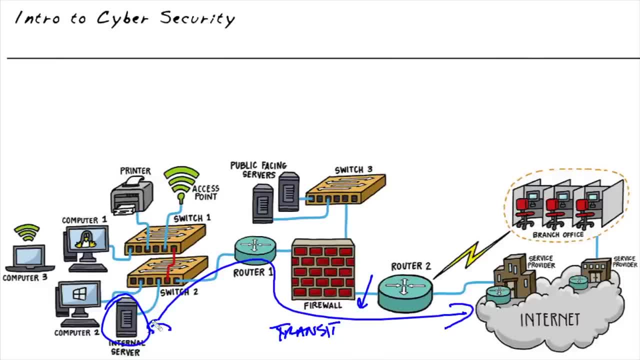 traffic and stealing the data. how do we protect it? And one big way of keeping that data, that information, confidential, so the unauthorized individual doesn't have to be able to see our sensitive or private information, is to make sure that the unauthorized individual can't read it or make sense of it, is to use encryption, which is 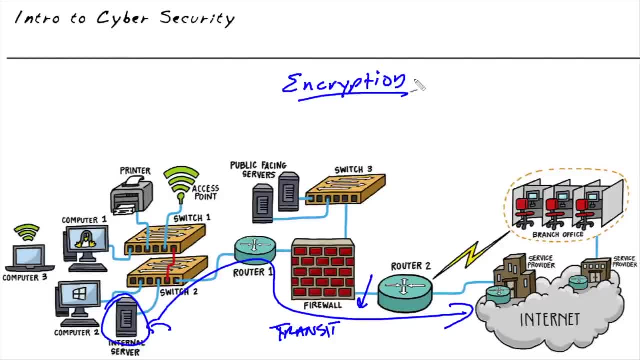 effectively scrambling the data so that the unauthorized people can't make sense of it, And popular methods of scrambling data in motion include IPSec, which is just an acronym. that means we're securing IP, and there's a whole bunch of rules that are set up behind that to make that. 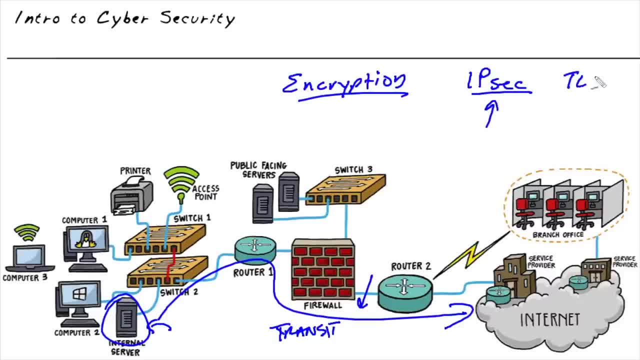 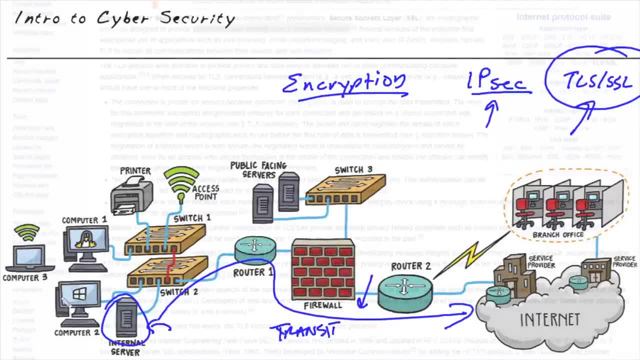 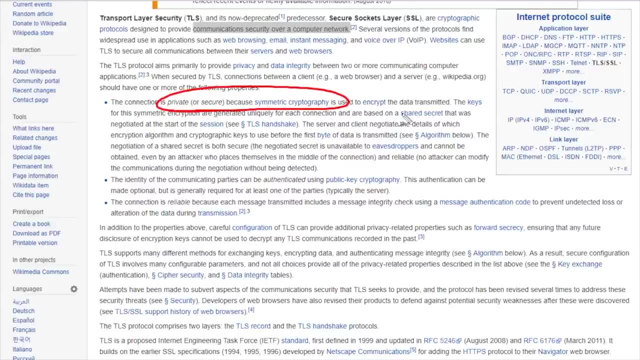 possible. Another one to protect data in motion is referred to as TLS or SSL, which is transport layer, security or secure sockets layer, and that's a very popular option that we use when we connect from a computer to a computer, Out to a website. that not only provides encryption and confidentiality, it also helps us to verify. 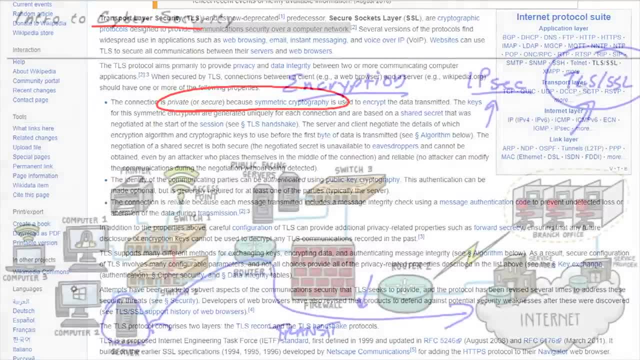 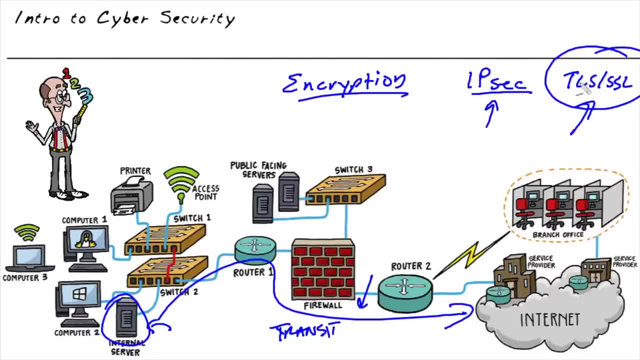 that we are talking to the correct site and not some hacker site. And then the third element that a company wants as far as protecting its resources and assets and doing good cybersecurity is to consider the potential compromises or attacks that might come up. And then, regarding those, 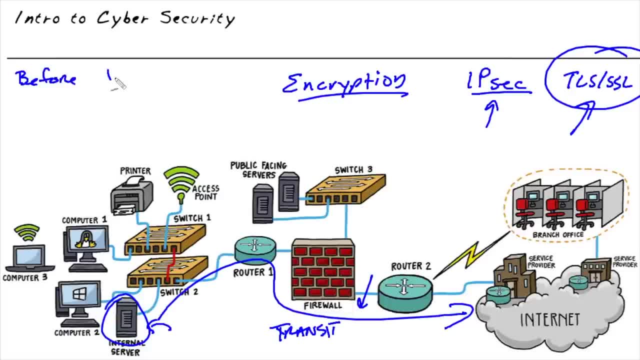 compromises, think about before, during and after, And part of cybersecurity is to consider the potential of the attack And then consider: okay, before the attack happens, what could happen, What are the vulnerabilities or weaknesses that each of our aspects of our system may have, And then put in. 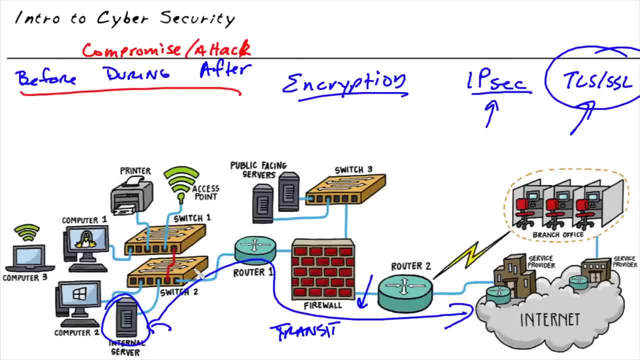 countermeasures or precautionary measures that can help prevent that type of attack from being successful. And, like my mom said, a stitch in time saves nine, And preventing an attack is way more desirable and takes a lot less time and effort than cleaning up after an attack. However, if attacks do happen, or compromises do happen, part of 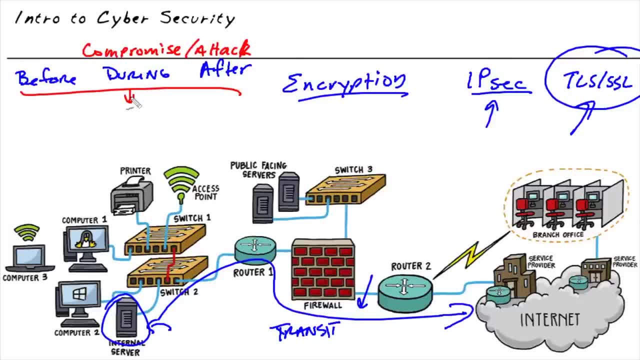 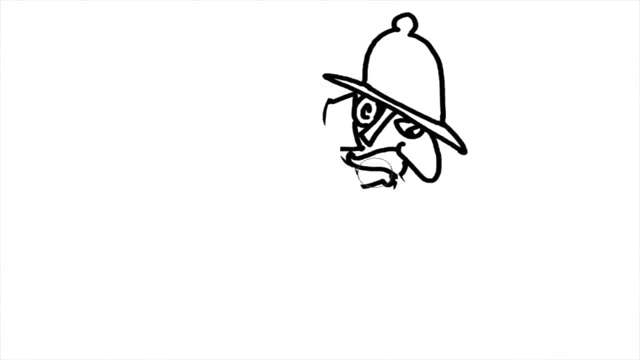 cybersecurity would be to respond to those attacks And that way the damage can be identified, contained, with the intent to restore full functionality and full security and also minimize the impact, the negative impact, of that security breach. And then, after an attack, there may be some investigations that are needed. So part of cybersecurity would be a well 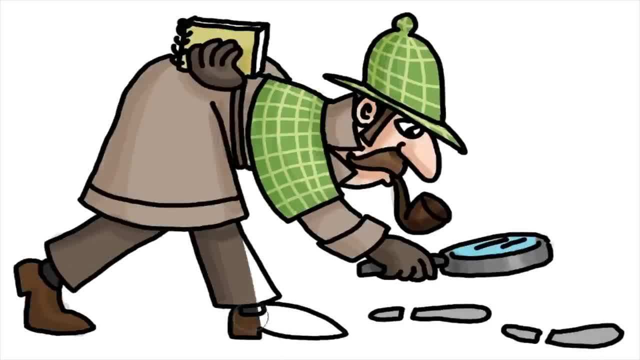 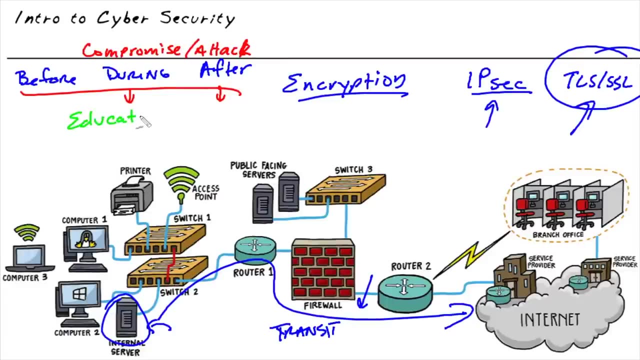 thought out plan of how we're going to do forensics and investigations regarding what happened, to clearly identify what did occur And the lessons learned from that would also be used to help prevent that type of an attack from happening in the future. And a huge aspect regarding cybersecurity is education. Wow, that's green. Green is a little hard to read. Let me read you that: 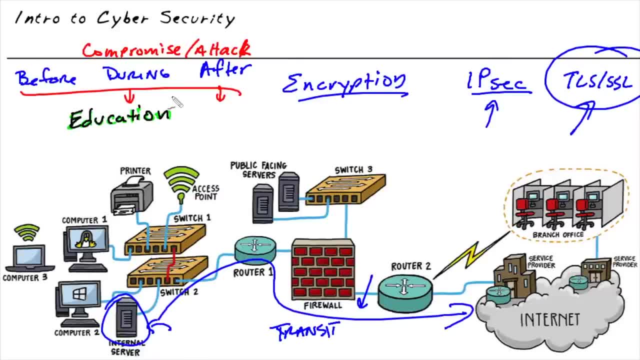 Education, Because a professional in the cybersecurity field is just one person or one team And there needs to be education across the board. Users are often the weakest link. Case in point: there may be a user here like Bob, And if Bob has, 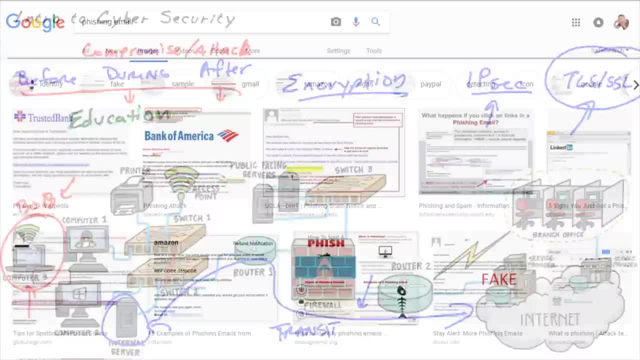 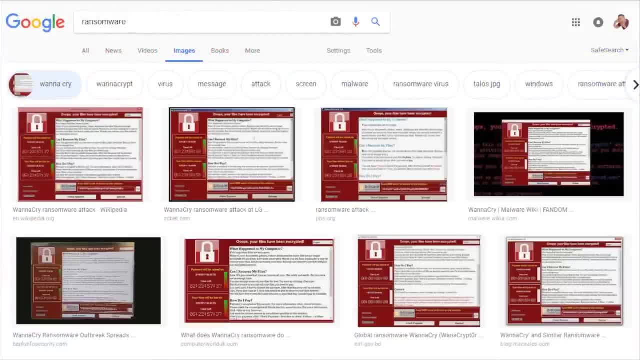 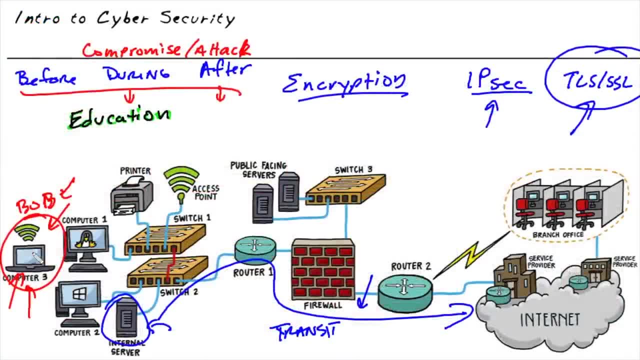 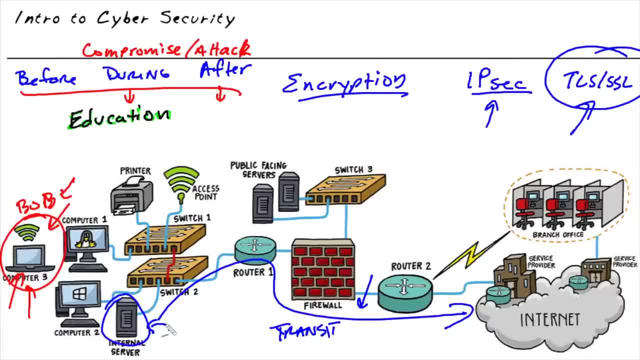 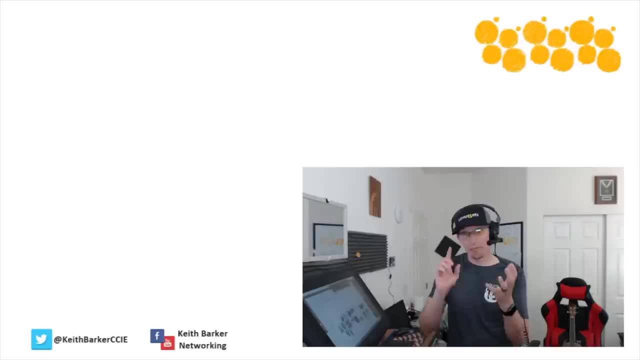 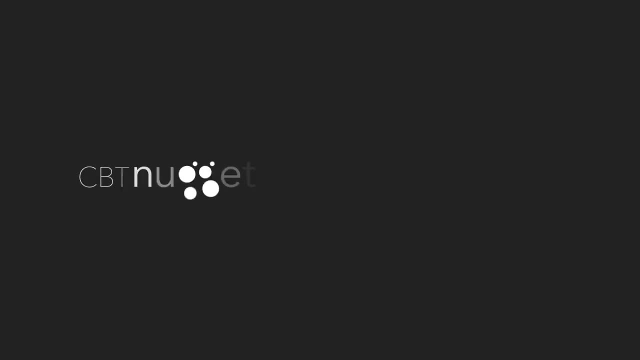 going to be able to do a lot of things. But he's going to be able to do a lot of things. 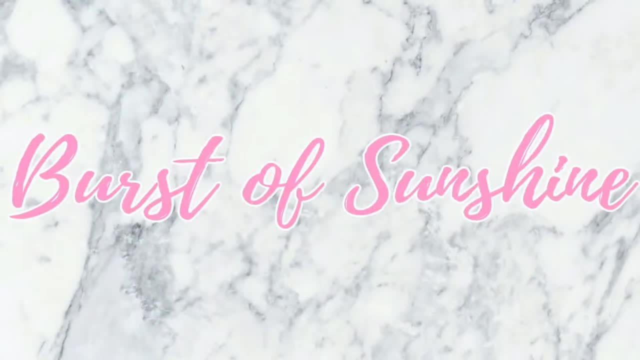 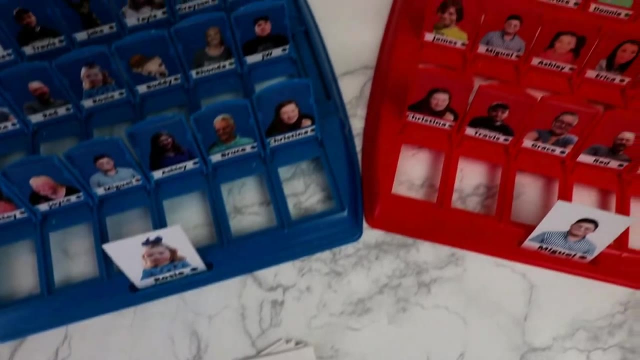 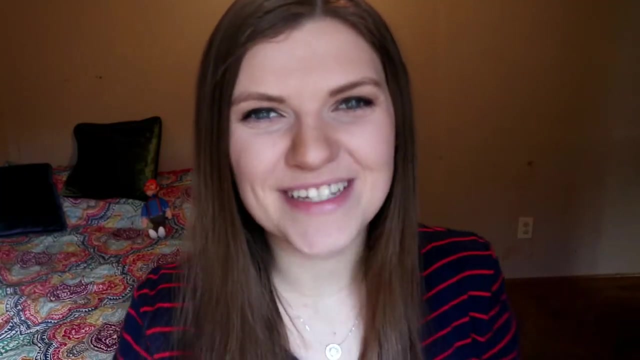 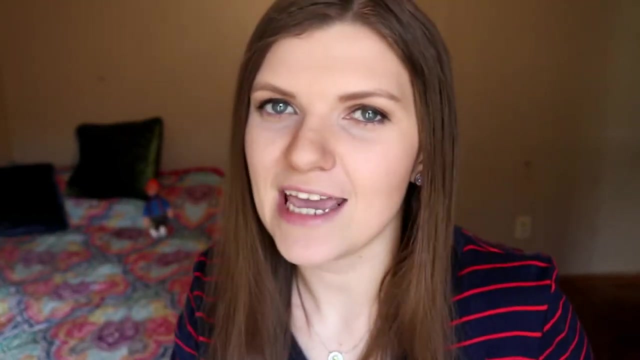 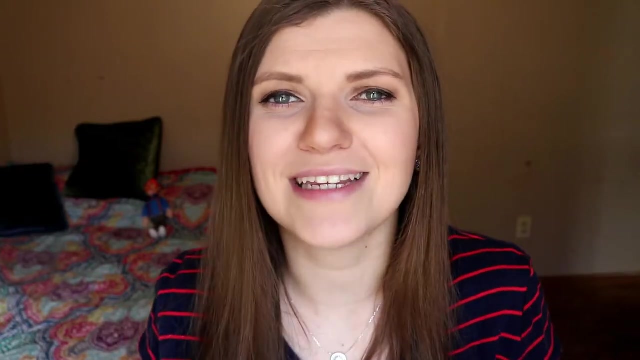 Hello there, Welcome to my channel, Versus Sunshine. I'm Ashley. In this video, I'm going to be showing you how I made another DIY custom game. If you've seen my Monopoly game that I made last year, it was super fun and it came out great, and I just love having a personalized board game to play. 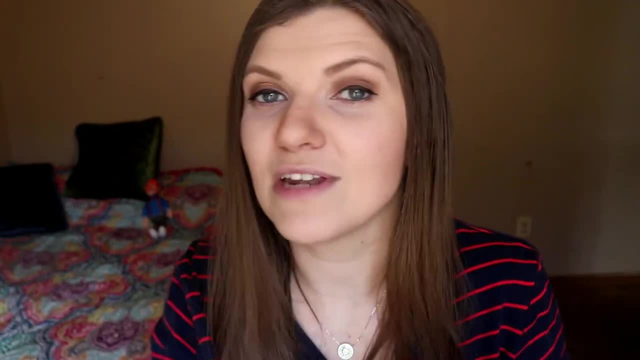 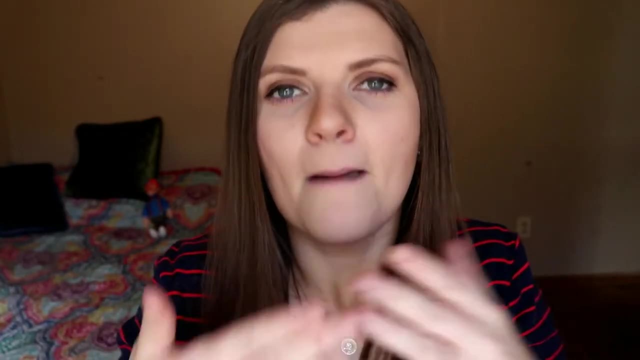 So I decided to spend on that, because the resolution of mine is that I would like to spend more time, you know, playing games and just spending quality time with my family, and a little bit less on our devices and a little bit more person-to-person interaction.